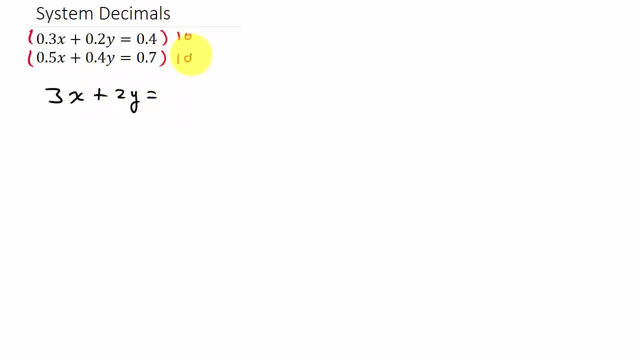 will give me 2y, and that, equals 10 times 0.4, would give me 4.. And then 10 times 0.5x would give me 5x, plus 10 times 0.4y would give me 4y, and that equals 10 times 0.7, which would be 7.. And now 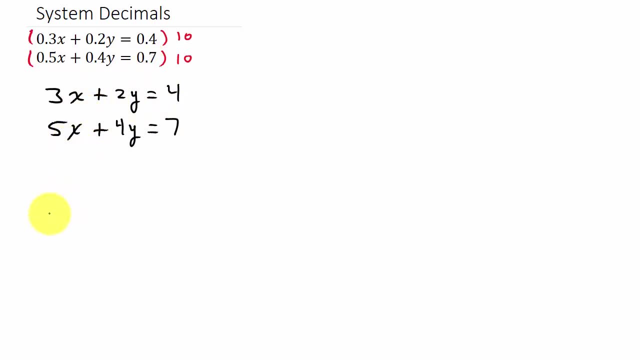 this is my new system, All right. so here we're going to use the addition method to solve the system here. So when I add the equations together, I want one of the variables to go out. So you can see, I could multiply the first equation by negative 5 and the second one by 3. That would give me 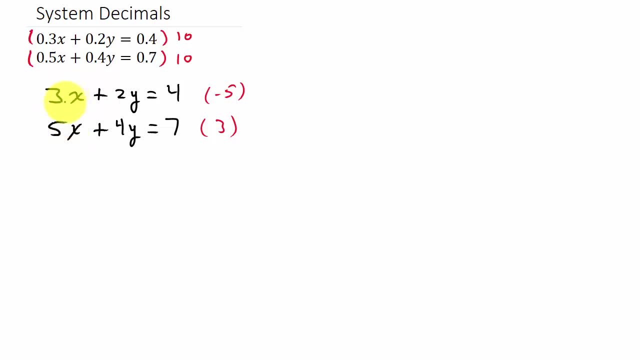 negative 15x and a positive 15x, and when I add, the x's would go out. And if I wanted to, I could multiply by negative 3 and positive 5.. That would give me positive 15 and negative 15. And if I add those together the x's would go out. But instead of multiplying each equation, 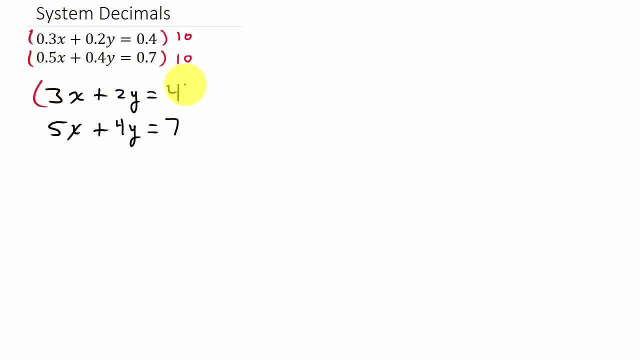 by a number. it would be easier just to multiply the first equation by negative 2, because that would give me negative 4y. So I would have negative 4y plus 4y. That would go to 0. Okay, but either way. 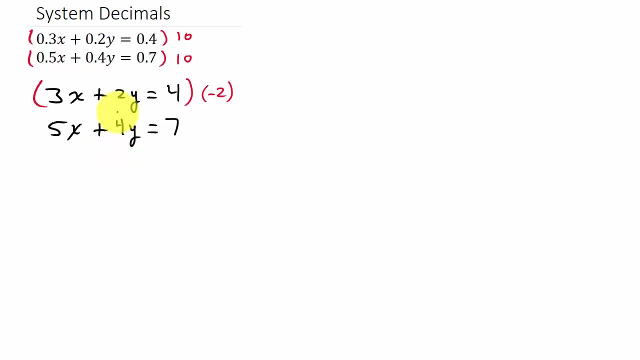 either one you do will give you the correct answer. All right, so if I do negative 2 times this first equation, Okay. so negative 2 times 3x Would be negative 6x, And then negative 2 times 2y would be minus 4y And that equals negative 4.. 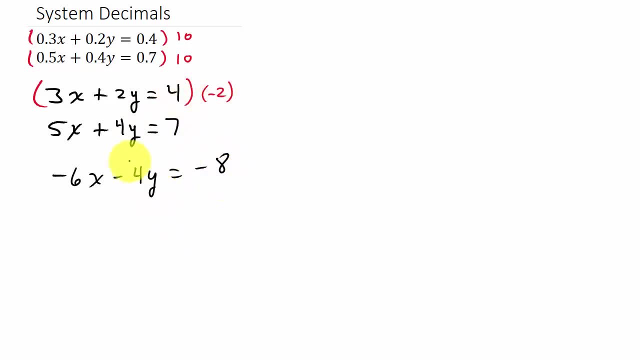 I mean negative 2 times 4, which is negative 8.. And then I didn't multiply the second equation by anything, So that's just going to be 5x plus 4y equals 7.. And then I add, And so 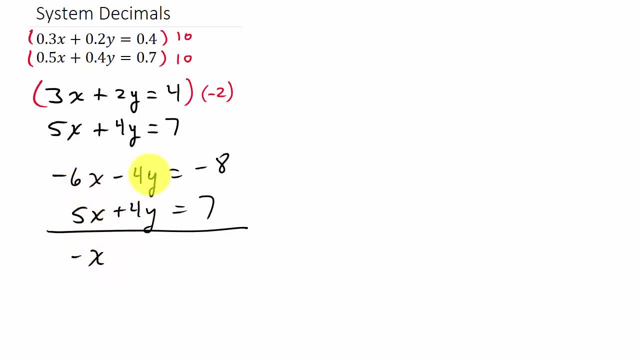 negative: 6x plus 5x is negative x. Negative: 4y plus 4y, that's 0. And then that equals negative. 8 plus 7 is negative: 1.. And now you can see I have negative x is equal to negative. 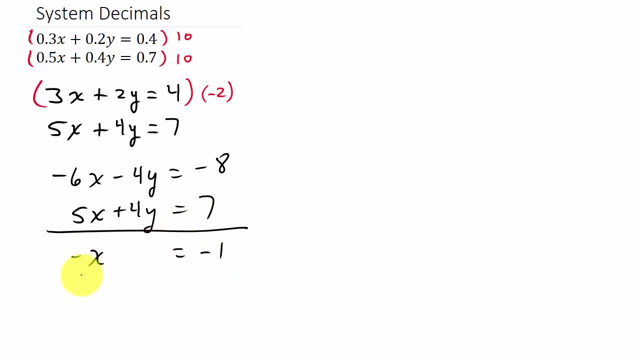 1.. So I'm going to solve for x by dividing both sides by negative 1.. And so that gives me x equals positive 1.. Okay, Now, remember, we've got to write our solution in the form x, y, And I already have my value. 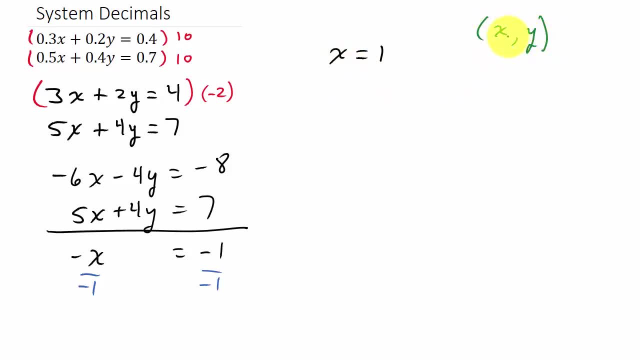 for x. So now I need to figure out what y is Now to solve for y. I can take my x value and I can plug it into any one of these four equations here. It makes no difference. So what I'm going to do is I'm going to take the negative 1 and I'm going to plug it into. 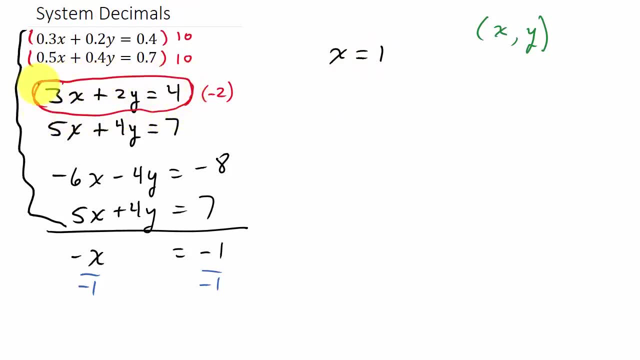 this one right here. and the reason: because the numbers are smaller, okay, and, like I said, you can plug it into any one. so let's plug one in for X. so I've got three times one. I'm putting one in the place of X plus 2y equals 4. so I've got 3 plus 2y equals 4, and then I'll subtract 3 to 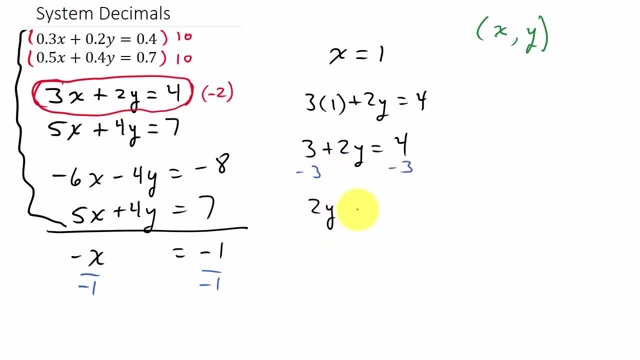 both sides, and so I get 2y is equal to 1, and then I'll divide both sides by 2, and so I get y equals 1 half, and so here's X, here's y, and I can write my solution in the form XY. so that's one one half is my solution. 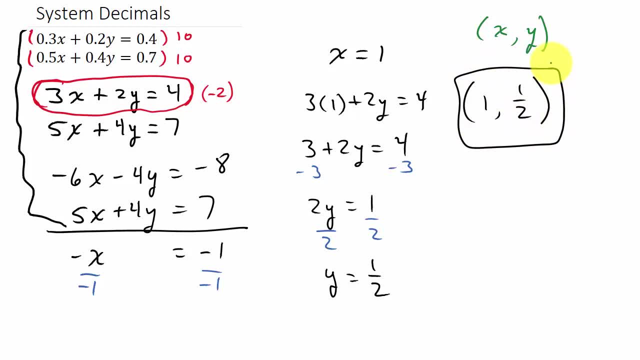 all right, so I hope the video helped check out my other videos. give me a like, share and subscribe, and thanks for watching.